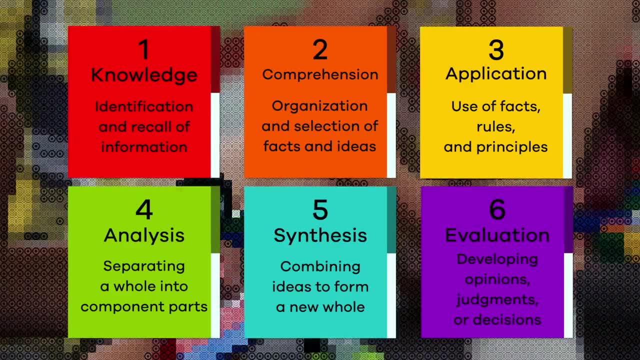 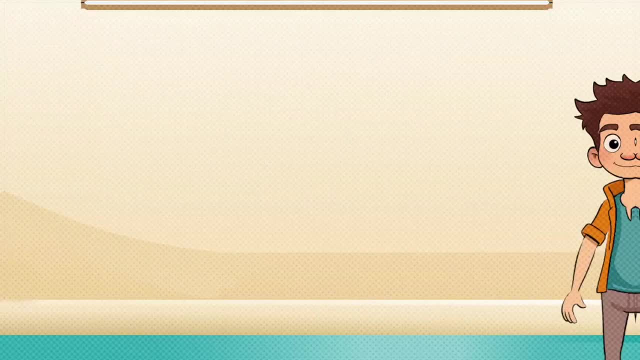 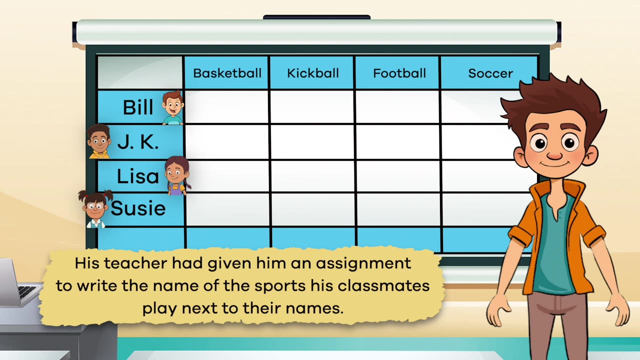 of the steps that we can use to help us. Okay, now let's put these skills to good use and help our friend Tyler out. Tyler has a problem. His teacher had given him an assignment to write the name of the sports his classmates play next to their names. 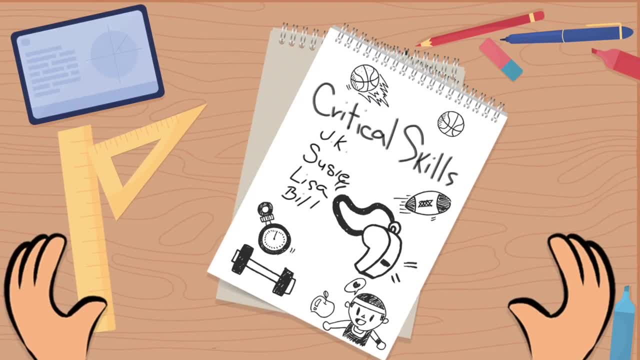 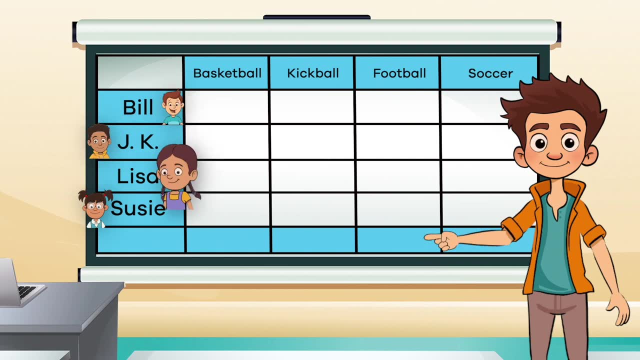 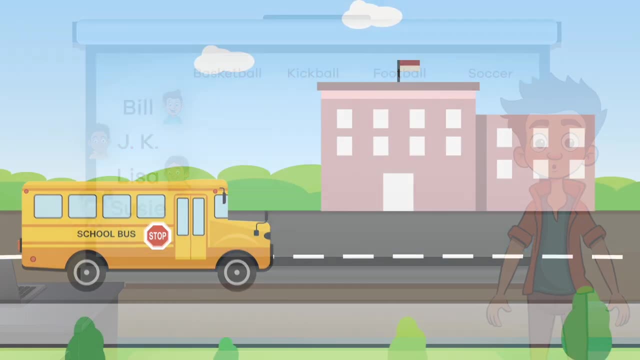 But Tyler didn't. He did not take great notes, So he has to remember what sports four of his classmates- Bill, JK, Lisa and Susie- like to play The worst part. He cannot ask them again because all of them are on a field trip. What a bummer, Since the assignment is due today. 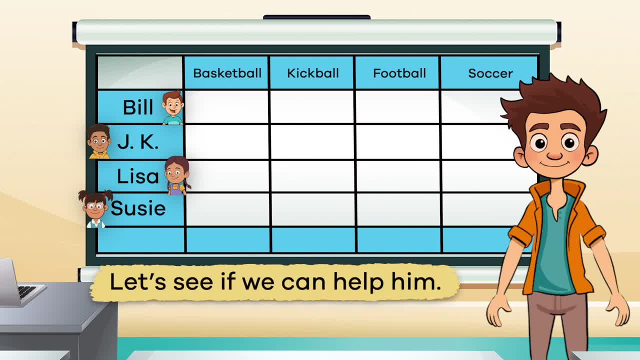 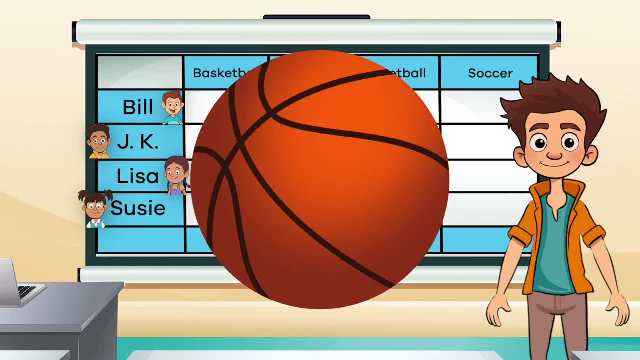 Tyler is running out of time. Let's see if we can help him. Let's start off with what information he needs to know about the sports he wants to play next. First up, there are the four sports he wants to choose from: Cyberpunk 2077, Presellt. 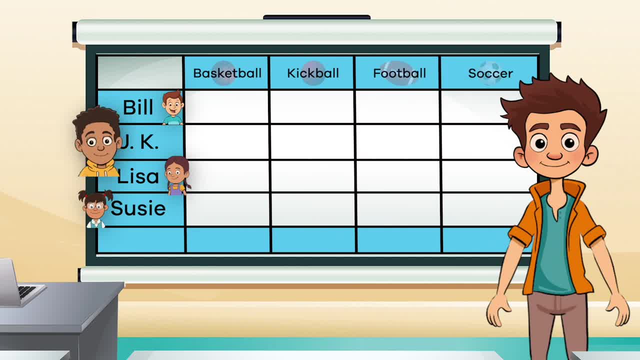 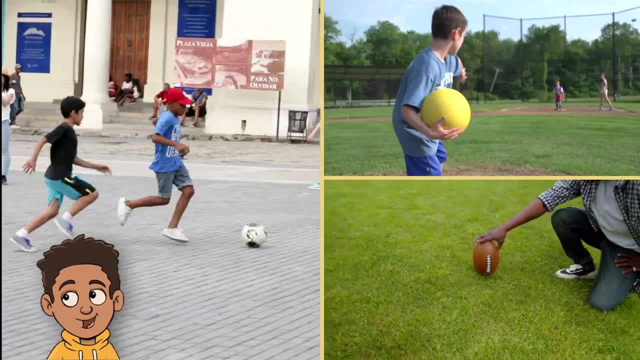 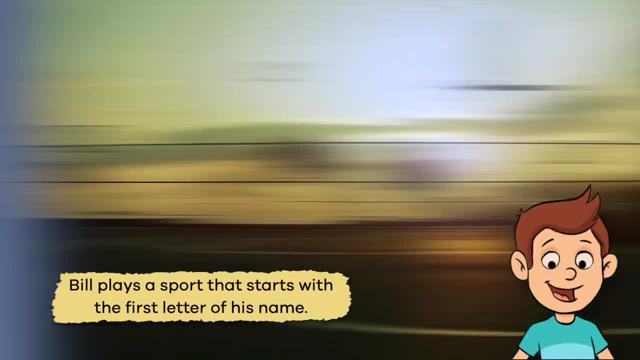 There are four sports he wants to choose from. He knows that JK thinks but doesn't like the kickball. He also knows that JK, Lisa and Susie don't play the same sport as Bill, And Bill plays a sport that starts with the. 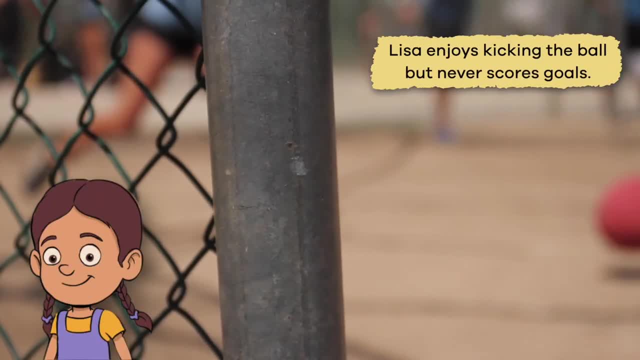 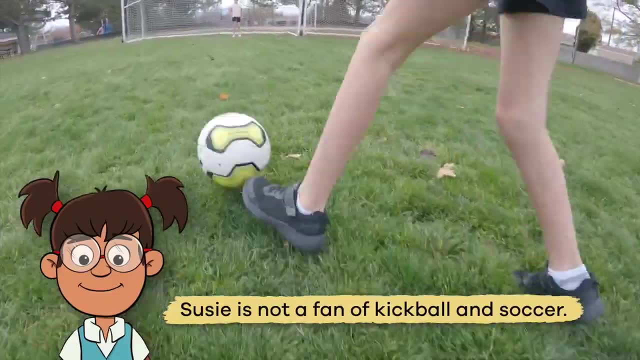 name It's. Can I Hope I Get Debut Day. It's Weber, An另外 4 Sport Especial. It's A chỗ for Bاح. My travels there Sk redundant, kicking the ball but never scores goals, And Susie is not a fan of kickball and soccer. 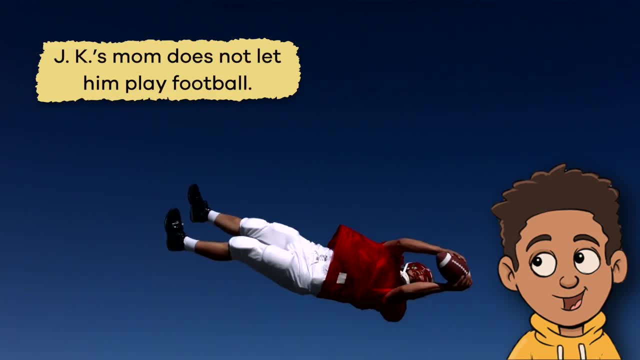 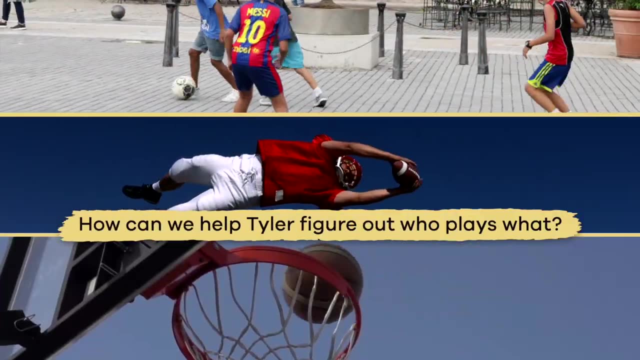 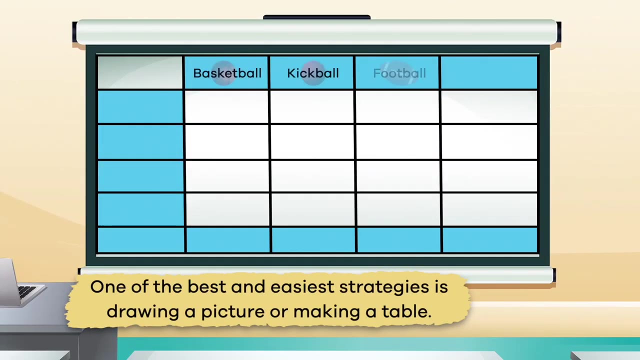 Oh yeah, and JK's mom does not let him play football. Whoa, that is a lot of data to consider. How can we help Tyler figure out who plays what? What are some strategies that he can use? One of the best and easiest strategies is drawing. 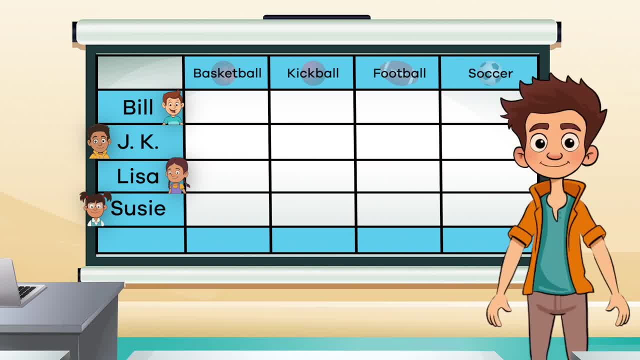 a picture or making a table like so. Tables are a simple way to organize information and help us narrow things down. Now that we have a table with the sports and classmates listed, we can consider the clues that Tyler has and draw an X every time an option is eliminated.